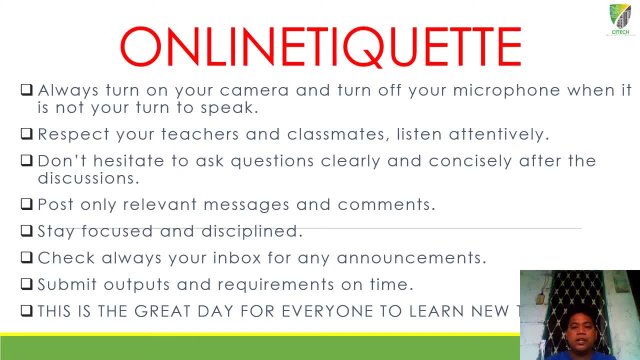 Okay, so we have here, first for us to be reminded, the online etiquette. The first one you have to remember is always turn on your camera and turn off the microphone when it is not your turn to speak. Number two: respect your teachers and classmates and listen attentively. 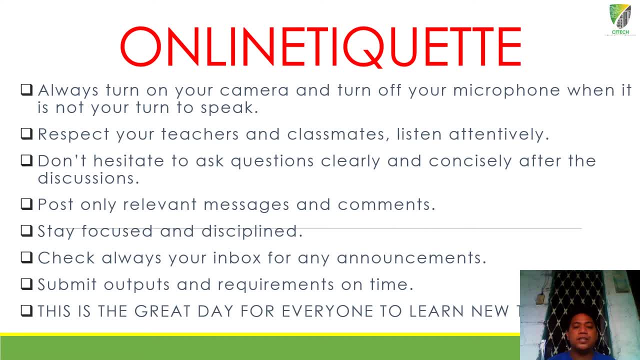 Number three: don't hesitate to ask questions clearly and concisely After the discussions. So for today, since we were going to have two parts- part one is the discussion and part two the question and answer portion- So if you have any questions regarding the topic, so just take down notes and after that, after my discussion, so in the part two, you may raise your question. 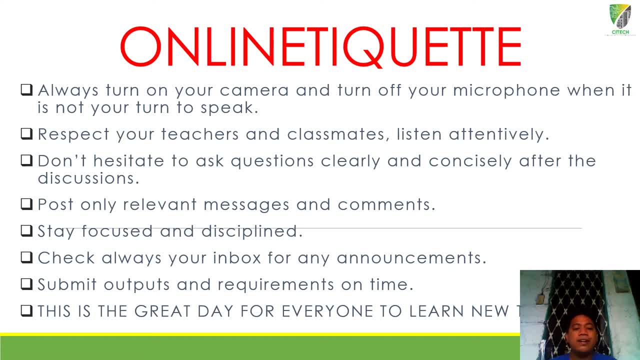 Next, online etiquette: post only relevant messages And comments. Five: stay focused and disciplined. Six: check always your inbox for any announcements. It's either in DGC or Microsoft Teams, But most of the time I am giving announcements in Microsoft Teams, since that is our major platform. 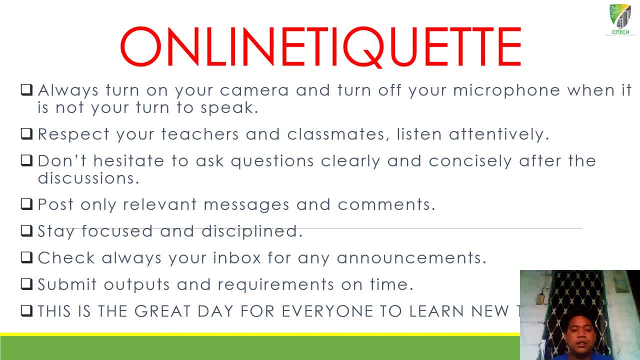 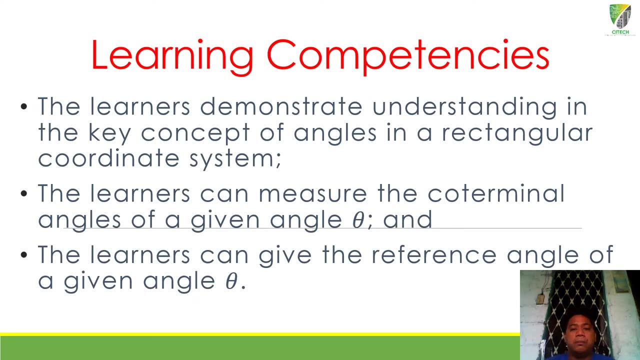 Next, submit outputs or requirements on time. next. so, since this is our great day for everyone to learn new things, so be excited and be amazed, thank you, and let us start our learning competencies. the learners demonstrate understanding in the key concept of angles and rectangular coordinate system. so kindly, 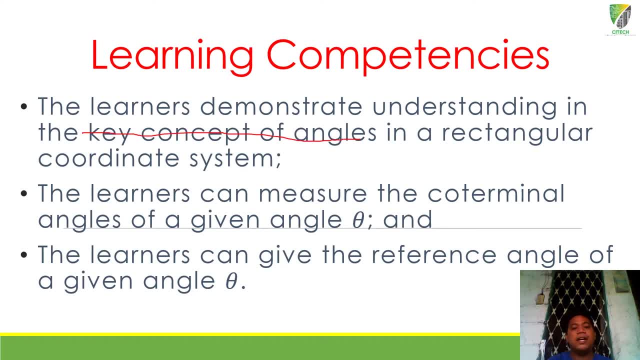 uh, be reminded about the key concept of angles. so that is our first topic and the second one: the learners can measure the coterminal angles, and the second one is the coterminal angles. next, the learners can give the reference angle of a given angle data. okay, so, reference angle. so 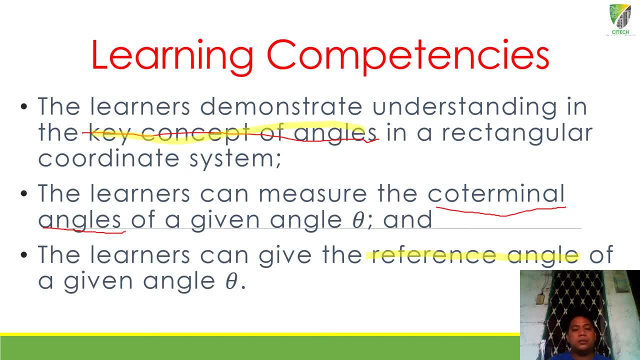 this. topics are being discussed along the journey of our teaching learning process. so the first one key concept of angles, the second one is coterminal angles and the third one is the reference angle. next, just a reminder to all of us, i am not here to entertain you. 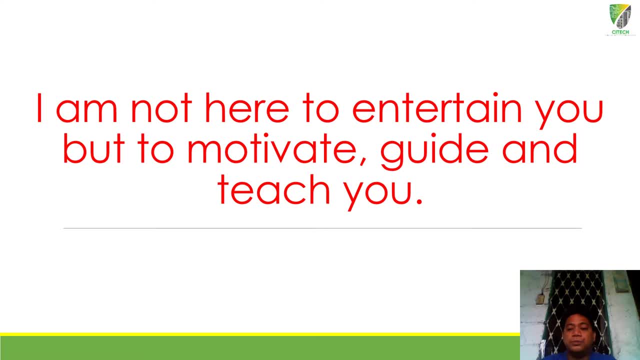 but to motivate by the teaching. okay, so i believe you know i will be serious in mathematics and trigonometry, but don't worry, this is not the negative portion of the uh subject. but i am here, uh, to guide you, to motivate you and to teach you, and sometimes i am giving a joke. 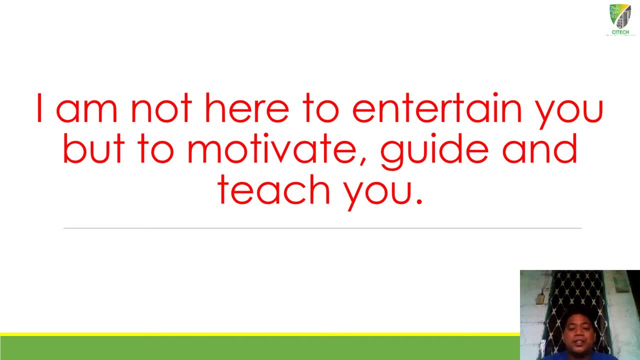 for that subject. but, um, it's up to you if you're going to love or not. okay, so that's it. so so, um, if you converted it as just an example for your feeling, you can send a message to the teacher if you strawberry, i want to get into this. 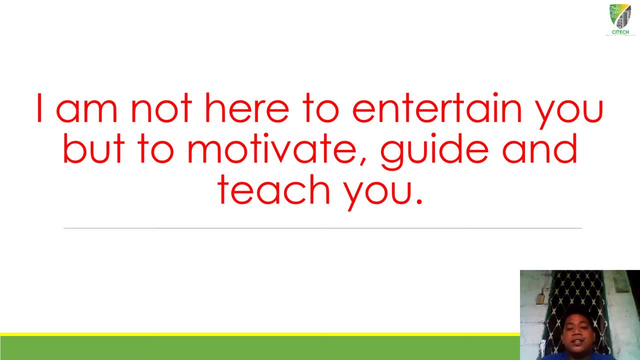 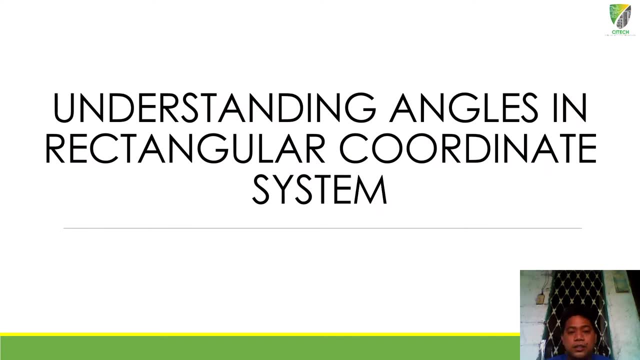 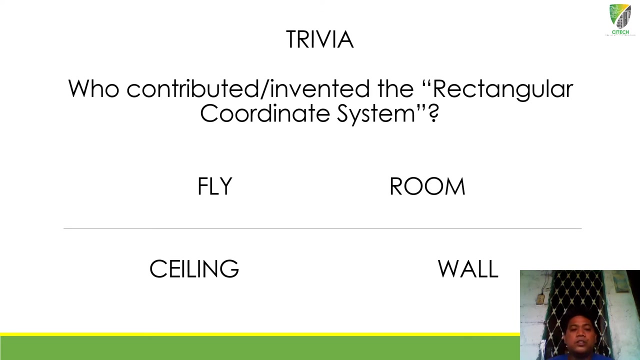 it's really easy at this point which is related to this topic. so first thing we have to understand in rectangular coordinate system is the angles. so the topic for today is the understanding, angles and rectangular coordinate system, coordinate system and we have here the trivia. so the first question in in our 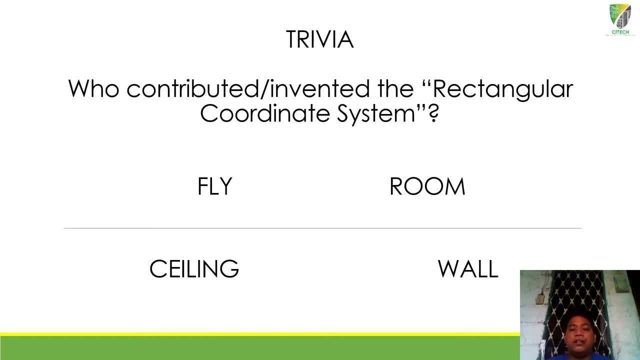 trivia part: who contributed or invented a rectangular coordinate system and what are the relationship about the word fly room ceiling wall? I have here this story about the rectangular coordinate system. okay, so the first thing we have to know first is that the coordinate system we commonly use is called the Cartesian. 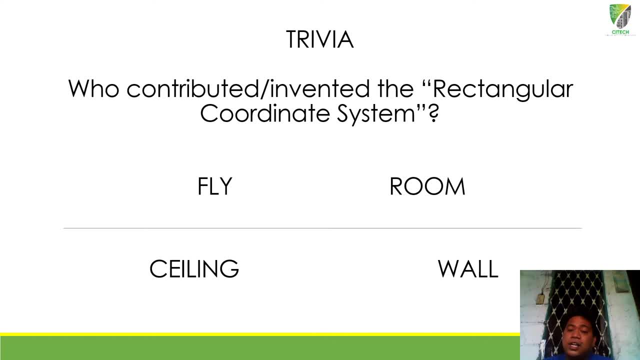 system after the French mathematics Rene Descartes. okay, right, the one who contributed or invented the rectangular coordinate system is no other than mr Rene Descartes, who developed it in the 17th century. legend has it that Descartes would like to stay in bed until late. was watching a film. 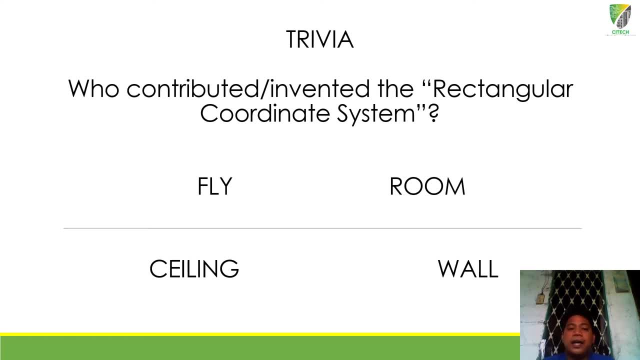 you know what I mean? he was lying on the ceiling from his bed. so from that time, mr Rene Descartes was in his room and after that he is lying on his bed. why? because he is sick. at that moment he wondered how to be the best describe the place, location. so while he 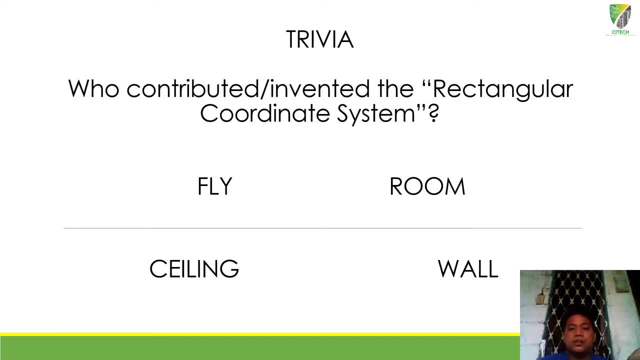 is lying in his bed. he looked at the ceiling. when he looked at the ceiling, he saw the fly, and after that he wondered how to be describe that- the location of the fly, where it is- and decided that one of the corners of the ceiling could be used as the reference. 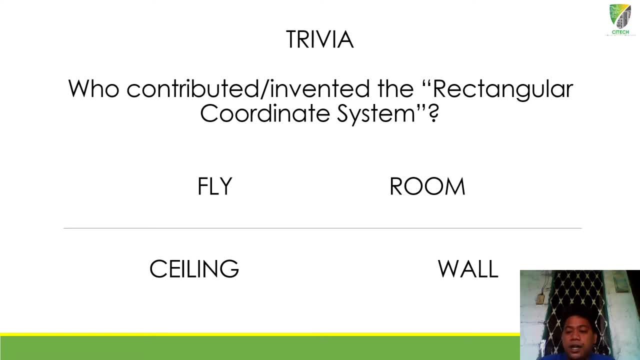 point. imagine the ceiling as a rectangular drawn on a piece of paper or a tool, as a two-dimensional. taking the left bottom corner as the reference point, you can specify the location of the fly by measuring how far you need to go in the horizontal direction and how far you need to go in the vertical direction to get to it. so for that moment, 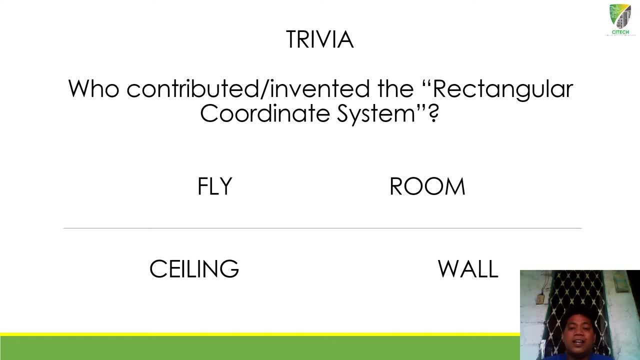 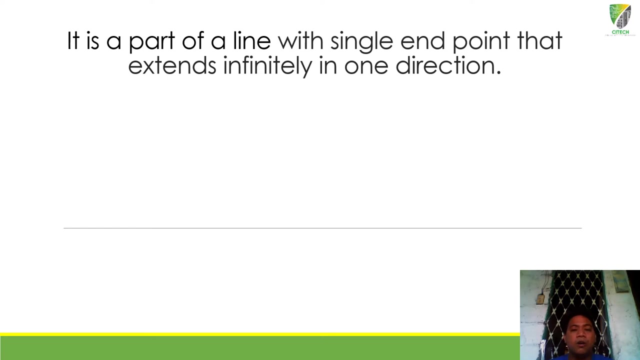 mr ledecore invented the, the x-axis and the y-axis, so from that, from that day on, he invented the rectangular coordinate system. so that is the. uh, that is the trivia for today. now let us go to our lesson proper. okay, so i will read first the definition and after that. so i'm going to. 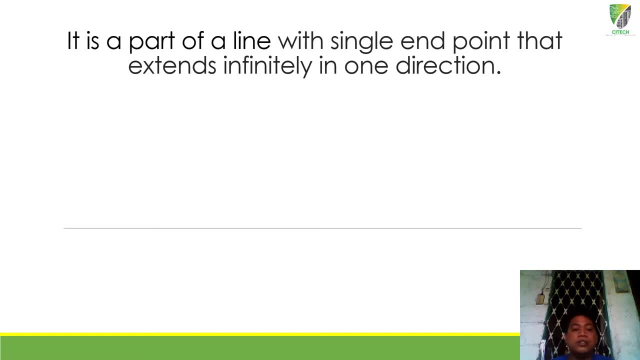 uh, give it to you the key concepts or the terminologies. so the first thing we have to know is to understand, or, uh, what i mean is to comprehend the meaning or the definition. so, for example, we have here- this is a part of a line, okay, so remember, excuse me, remember the word. 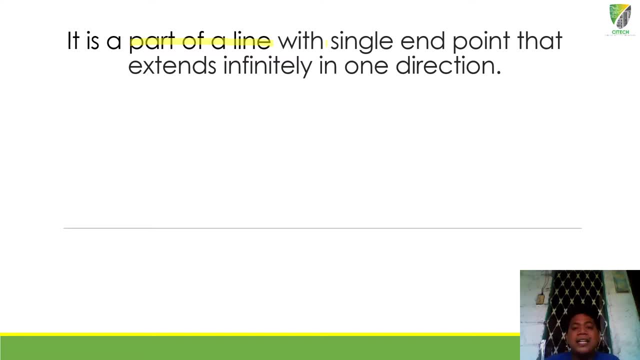 part of a line with single and point that extends infinitely in one direction. so from that, key terms or keywords. so i think you have the idea already: part of the line that has single end point and extends in one direction. yes, that is a ray. so the ray has. 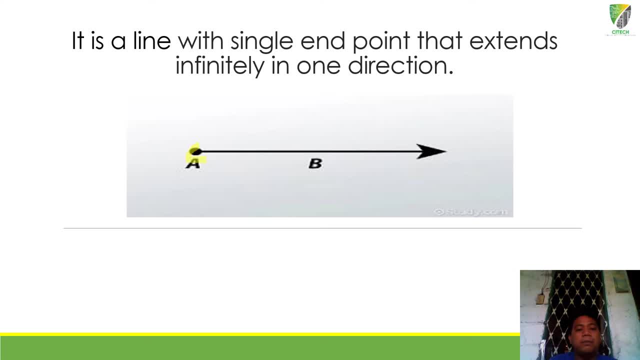 or it is a part of a line and has one end point extending in one direction. i'm sorry for the the uh curved line. so actually that is a line, so that it was a straight line. okay. so sorry for that curved line. so next, that is what we call the ray, okay. so next it is formed when two rays meet. okay. 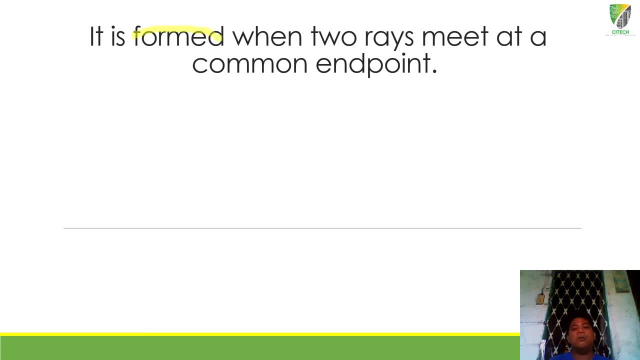 so it was formed when two rays meet at a common end point. okay, so let us have the common end point. so that is, we have here the ray one, ray two and the common end point, which is the vertex, and that is called the angle. so that is the forming of two rays meet at the common endpoint. 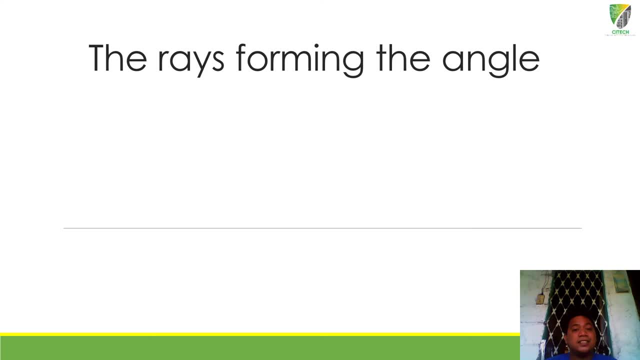 next, this is the race forming the angle. so what do you call that race that forms conangel? so that is what we call the sign. next, this is also the point at which the race meet. so what do you call that point that the race meet, or where the two race meet, or the two or more race meet, and this is what we call the vertex. 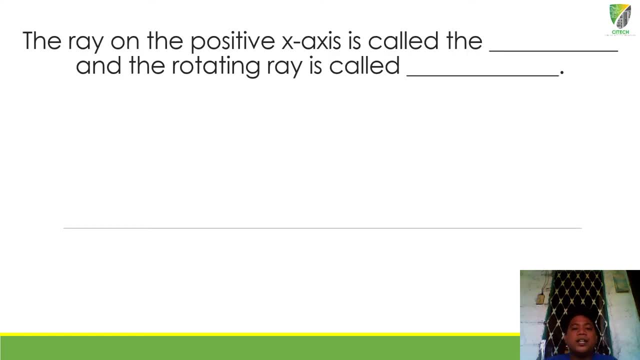 next, the ray on the positive x axis is called the blank and the, The dictating ray, is called black. So we have here the figure. So, as you can see, we have here the initial site from the positive x-axis, That is, the ray of a positive x-axis. 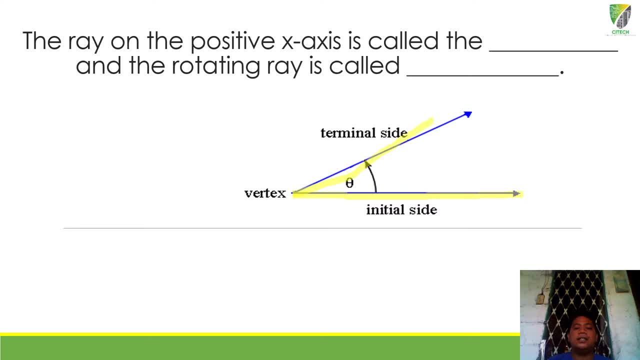 And this one is the terminal site. So, given that the ray on the positive x-axis here is what we call the initial site and this one, the rotating ray, is what we call the terminal site, Why is it called as the rotating ray? 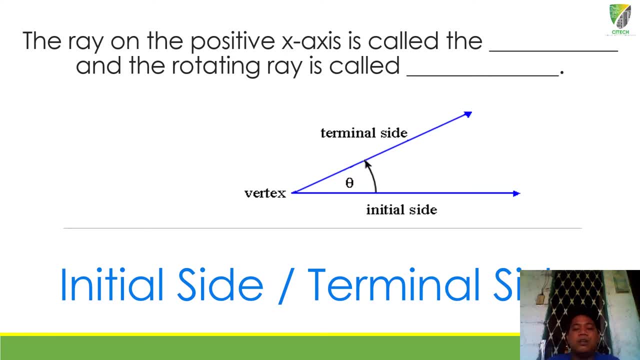 So why is the terminal site called as the rotating ray? So, since we all know that the terminal site can go in the direction, direction of every direction in quadrant 1, or terminal site can be here in quadrant 2, or can be here in quadrant 3, or can be here in quadrant 4.. So it means simply, terminal site is also called as the rotating ray. Okay, next, If the terminal site of an angle in standard position coincides with one of the axes such as 90,, 180,, 270. or 360 degrees, it is called the quadrant angles. 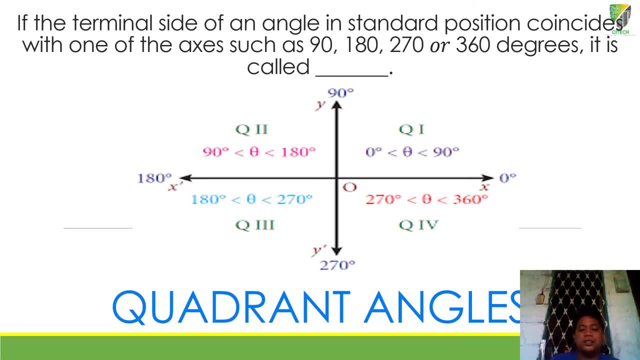 Why is it called as quadrant angles? Because this 90 degrees is right there on the y-axis And the 180 degrees is right there on the x-axis. The 270 degrees is on the y-axis And this is 0 degrees, because this is the starting point. 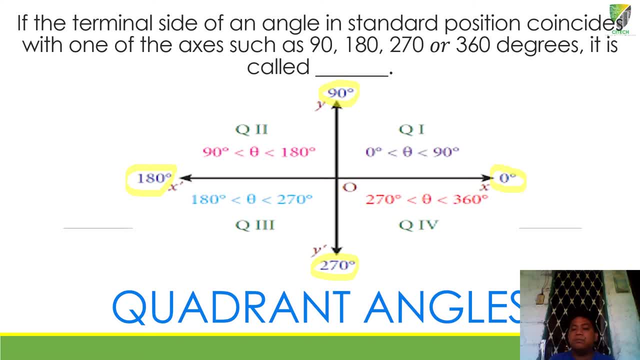 Or the starting angle, But most of the time it is 360 degrees As symbolizing as one revolution. So 360 degrees, Okay. So we have here the quadrant. 1. 0 degrees is less than the angle. Theta is less than 90 degrees. 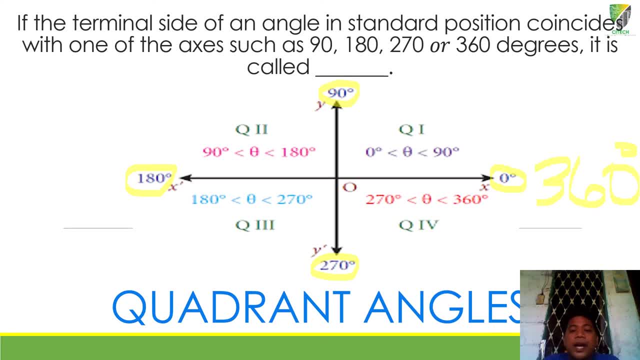 It means that starting from 1 degree to 89 degrees, So those Angles belong to quadrant number 1.. Again, 1 degree to 89 degrees belongs to angle at quadrant number 1.. And quadrant number 2.. 91 degrees to 179 degrees belongs to quadrant number 2.. 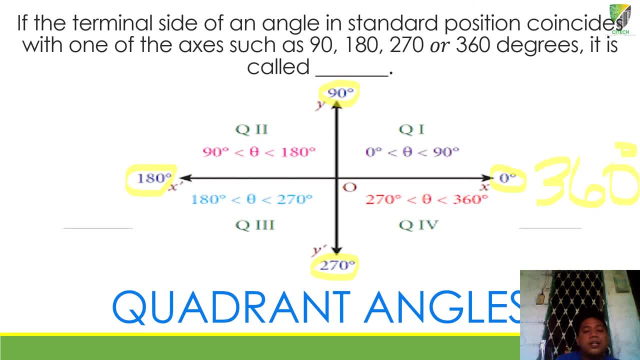 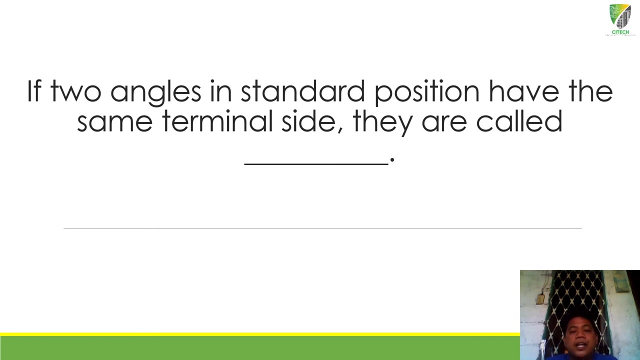 181 degrees to 269 degrees belongs to quadrant number 3.. 271.. 271 degrees to 359 degrees belongs to quadrant number 4.. So that's it. Next, If two angles in standard position have the same terminal side, they are called coterminal. 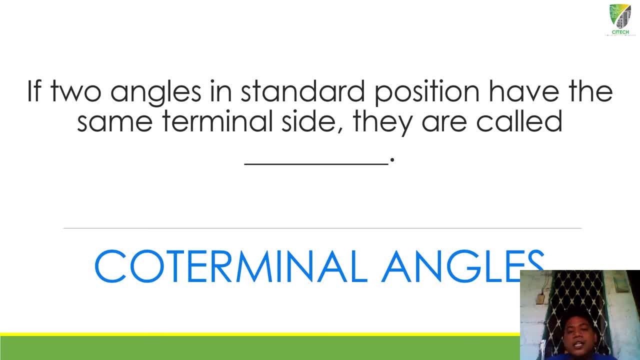 angles. Okay, So lay at the long journey of our discussion for today. So I will be discussing more about coterminal angles. So I will be discussing more about coterminal angles. So I will be discussing more about coterminal angles. 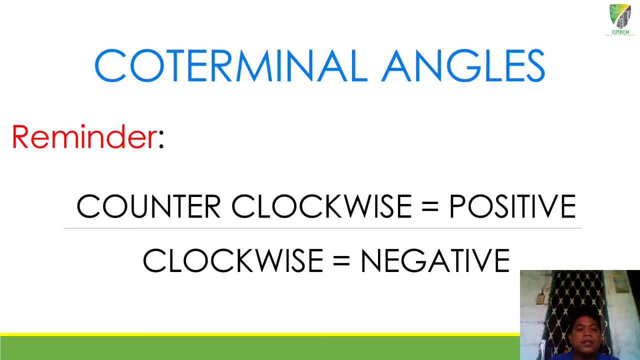 Since this is our second topic. Next, coterminal angles. This is just a reminder: Counterclockwise is equal to positive And clockwise is equal to negative. So, for example, we have here, like this, Y-axis and this is the X-axis. 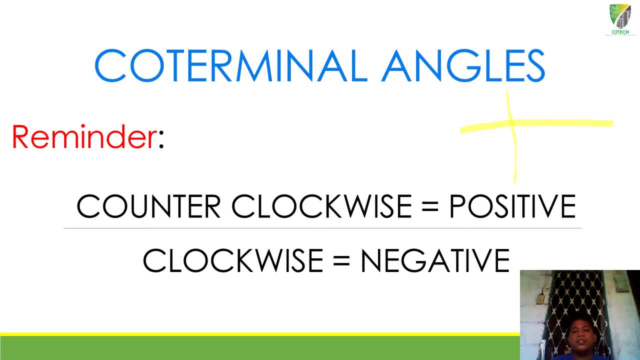 So if you are going to move the direction counterclockwise, like this one, It means that was a positive. But if you are going to move the terminal side into a clockwise moment or clockwise direction, it was negative. So be reminded of that because we need that in the next lesson. 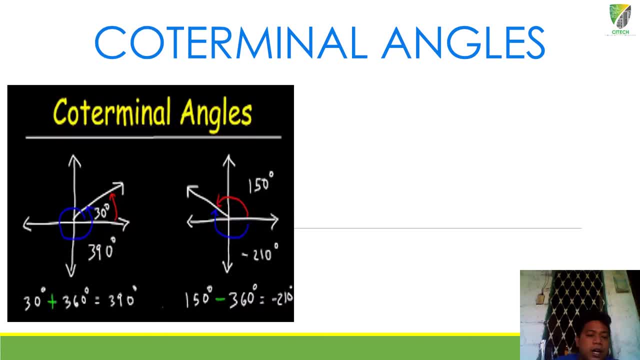 Next coterminal angles. So, for example, we have here, So we have here the example, which is 30 degrees angle. So this is the initial side and this is the terminal side And this is the sample or given angle. So the red one or the red arrow represents the counterclockwise. 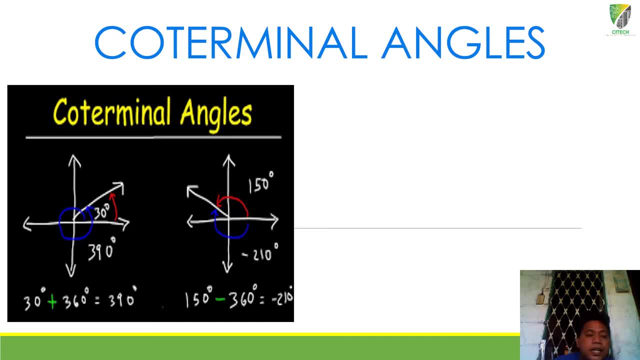 It means this is positive. So from the initial side up to the terminal side. So this is a Positive, since counterclockwise style, So 30 degrees. So this one, the blue arrow, from the initial side up to one revolution, up to the terminal side. 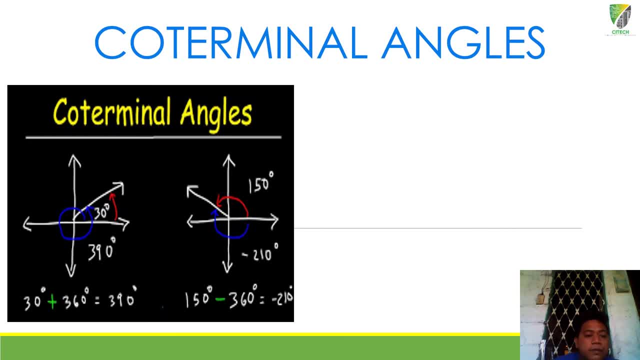 It has 390 degrees. Why So? from here, from the initial side, up to here, So 180 degrees, up to here, 270 degrees and up to here is 390.. 360 degrees plus the 30 degrees to terminal sides, to the equivalent of 390 degrees. 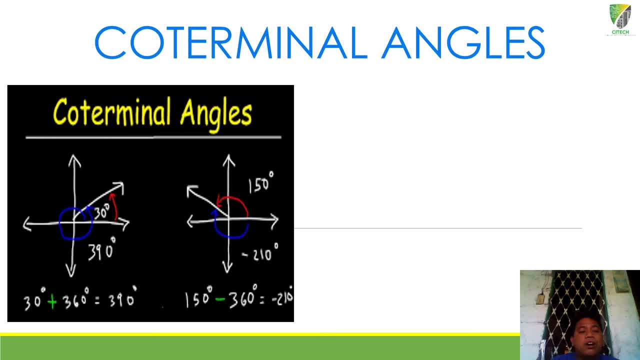 So now, what is the relationship of 30 degrees and 390 degrees? And that is what we call the coterminal angles. Why? Since they fall together in the terminal sides, Since they are both angles, So it means They are called coterminal angles. 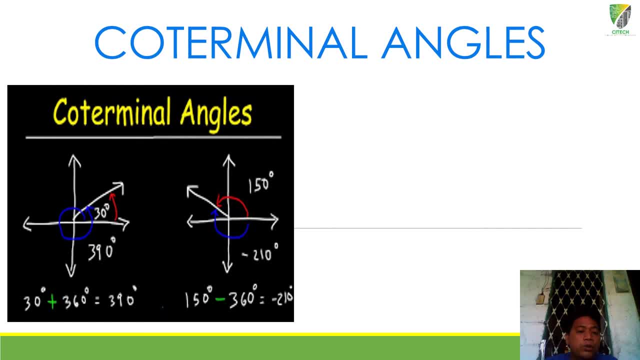 Since they fall, or they fell both in the terminal sides. Next, The figure number two: here the red arrow, is the counterclockwise direction. It means this is positive. So example: we have here the given 150 degrees and this one, the blue arrow. 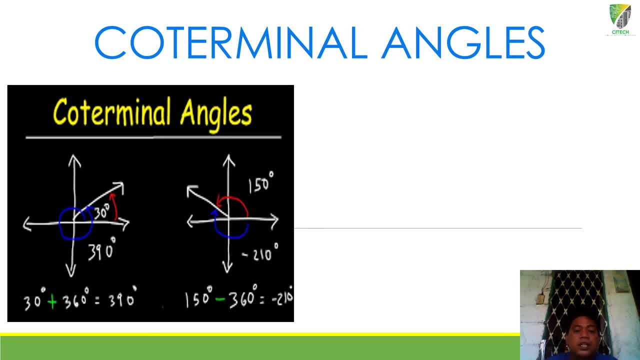 Since counterclockwise, Since clockwise direction, So it has a measurement of negative 210 degrees. Why? From here up to here, So we have here negative 90 degrees. Why negative 90? Because it moves the direction of clockwise. 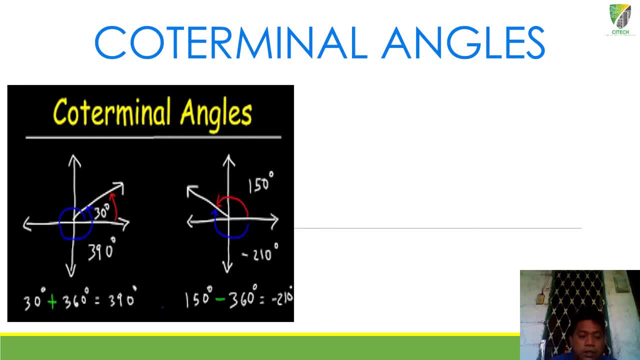 So here to here, we have here negative 90 degrees, up to here Negative 180 degrees, And since we all know that this is 150 degrees, So the remaining angle here is 30 degrees. So from here to here, negative 180 plus negative 30 degrees. 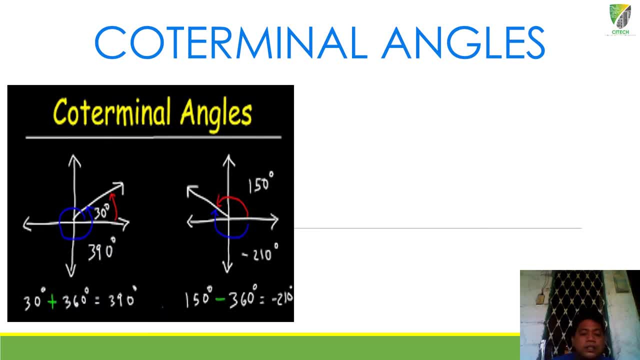 So that is negative 210 degrees, Or simply just subtract it from negative 360.. Since we have here 150 degrees, the given, So if you're going to get the another turn for terminal side, So since we have here And why we have here negative 360 degrees, 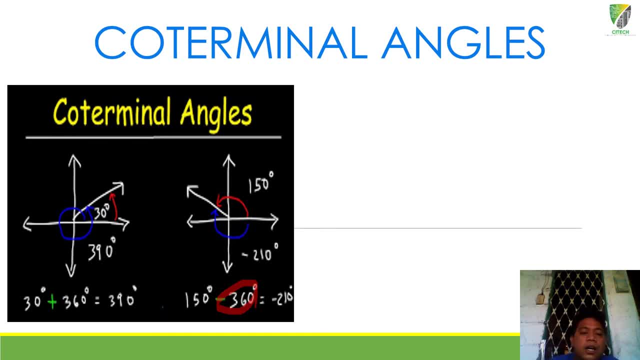 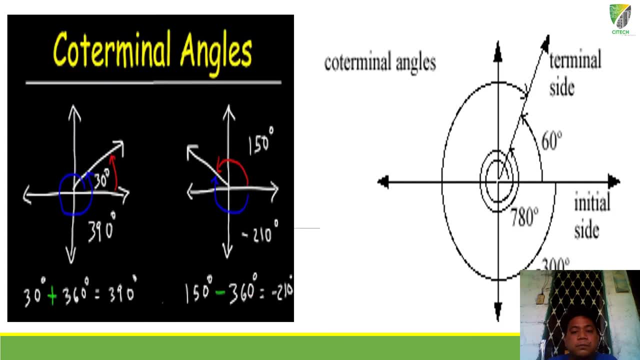 Because one revolution from here Up to here, So that is 360 degrees. Next, Another example: From here, initial side, up to here, the terminal side, So this is the given 60 degrees. This is positive because of counterclockwise direction. 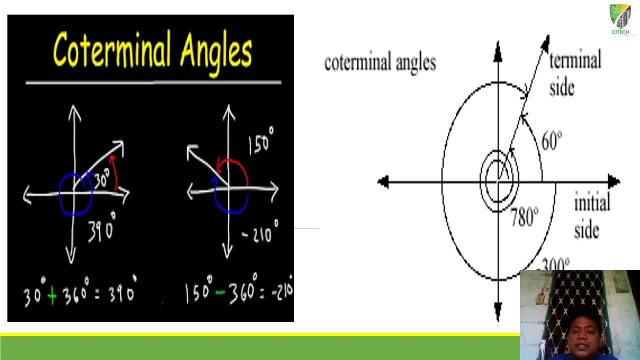 Next one. So from here, initial side, the another angle, we have here the first revolution. So it means 360 degrees. Another revolution, 360 plus 360 is 720 degrees, And up to here for the terminal side to get the terminal angles. 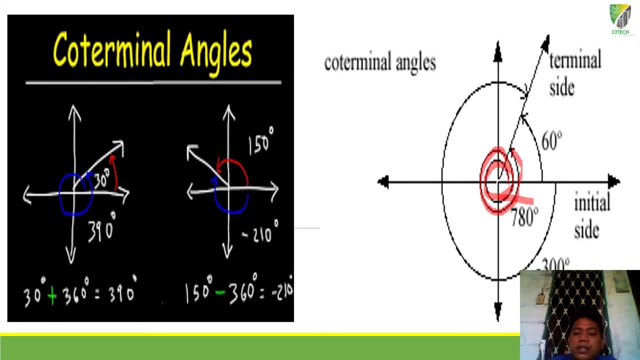 So 720 plus 60, we have here 780 degrees, And also from here up to here, so negative 90 degrees, up to here So negative 90 plus negative 90.. So that is negative 180, up to here negative 270.. 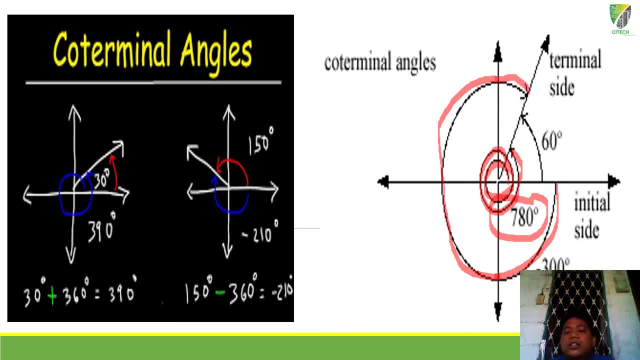 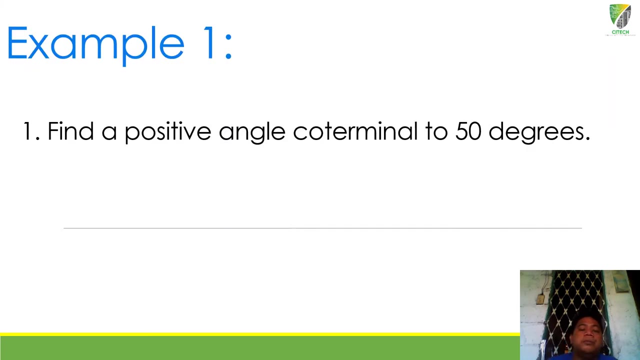 Since we have here another negative 30 degrees, So negative 270 plus negative 330.. So a total of negative 300 degrees. So it means that 60 degrees, 780 degrees and negative 300 degrees means they are coterminal to each other or they are coterminal angles. 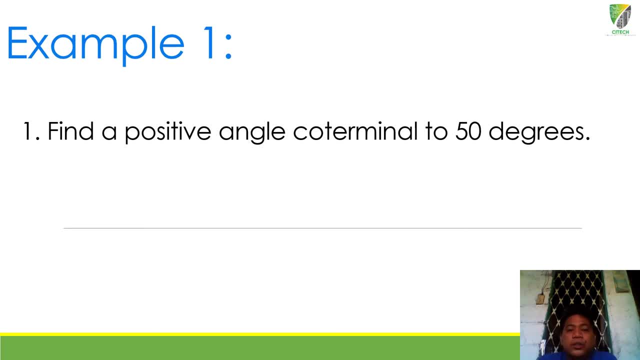 Example number one: find a positive angle coterminal to 50 degrees. So we are going to find a positive, Positive coterminal angles to 50 degrees. So simply just add 360.. Why? Because one revolution to terminal side is equal to 360 degrees. 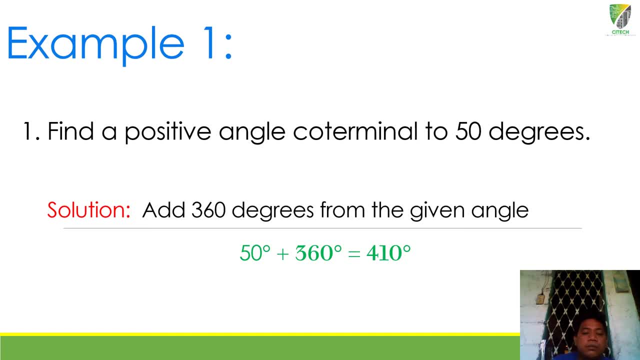 So since we have the given angle, which is 50 degrees, we have here just add 360 to get the positive coterminal angle. Just add the two given. So 50 degrees plus 360 degrees, we have here the total of 410 degrees. 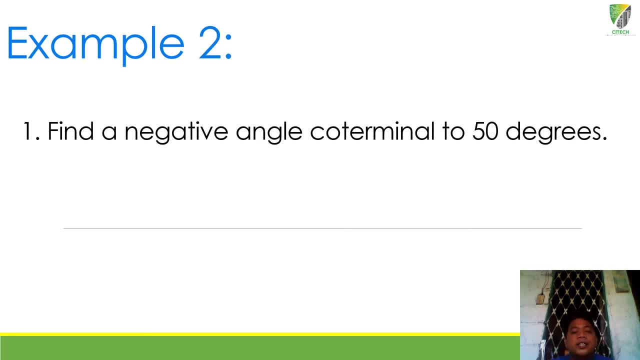 Next, if you are going to find the negative angle coterminal to 50 degrees or any given angle, so just subtract. So if earlier the positive angle, I just add 360.. Here in negative angle. so if you are going to find it, so just subtract 360 degrees. 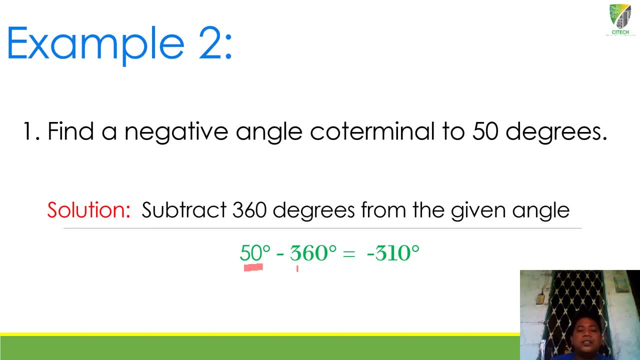 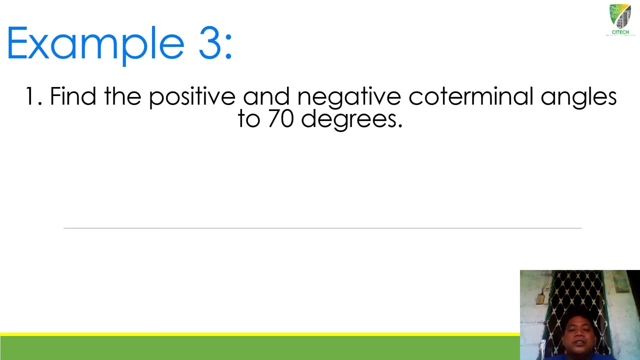 So we have here: the given 50 degrees minus 360 degrees is equal to negative 310 degrees. So that's it, Just. it's just as simple as a piece of cake. Next, find the positive and negative coterminal angles to 70 degrees. 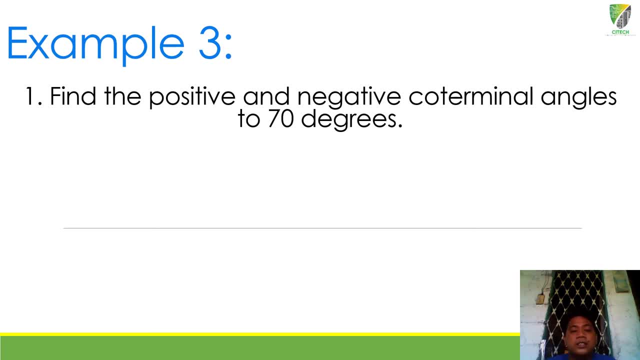 So we have here the given angle, 70 degrees, So for you to have the positive and negative coterminal angles of it. so just in a positive, just add 360.. Positive, just add 360.. If you are going to get the negative coterminal angle, 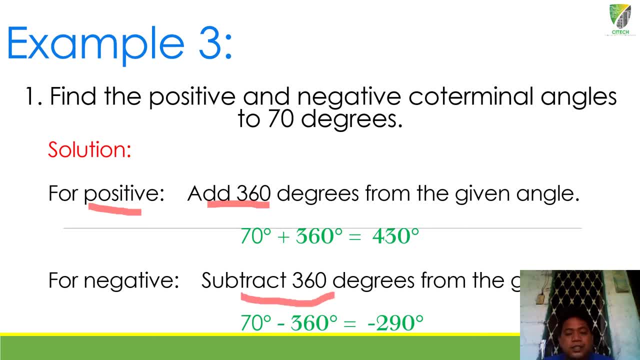 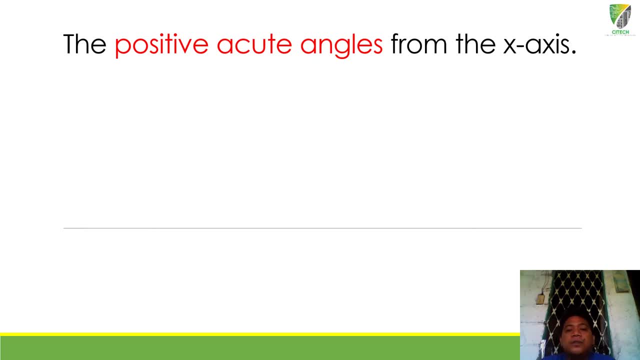 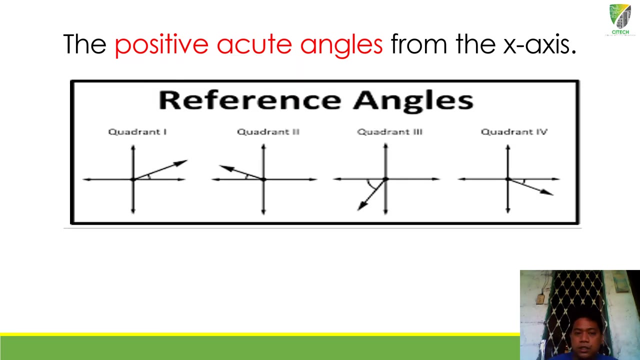 Just subtract 360.. So that's it. It's just as simple as a piece of cake. Next, positive acute angles from the x-axis. Be careful, or just be reminded that this the word positive acute angles. Why Like this? 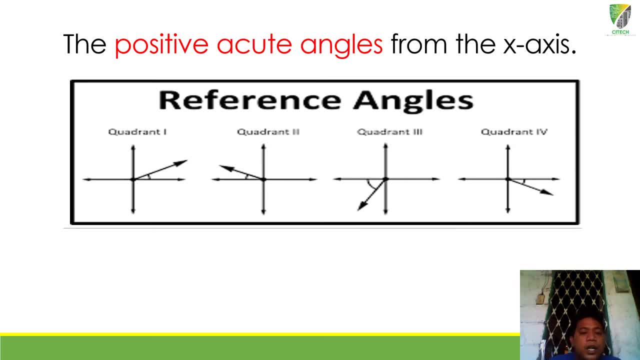 So reference angle: we have here the quadrant 1.. So since we have here the terminal side in the quadrant 1, so maybe it it measures 30 degrees, So this is already positive. Okay, So be careful. sa word na acute. 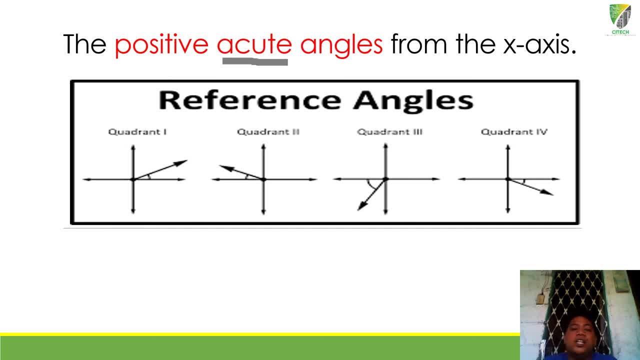 Okay, So kapag right angle ang naproduso mo, so hindi siya magiging reference angle na tinatawag. This is our second topic: reference angles. So be careful ng sinasabi natin dito ay Acute angles and positive. 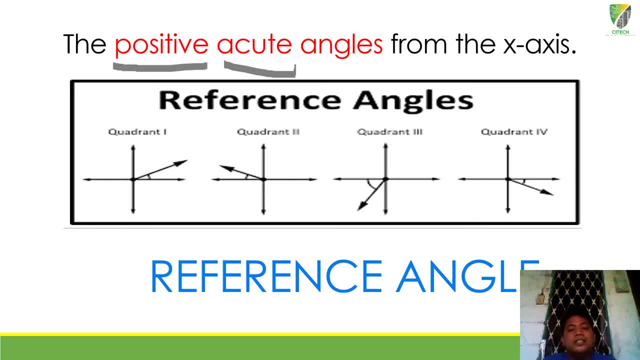 Paano, sir? kapag hindi yung negative, It's okay, Just get the absolute value of that angles and find the acute angles of that. So paano kaya yung sir? Okay, So we have here again sa quadrant number 1, kung mapapansin natin, 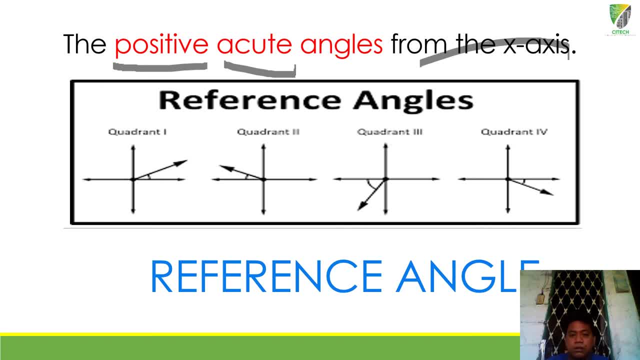 Be careful. Sabi ko nga. So let us erase first. Okay, So be careful sa ating definition for reference angle, So the positive acute angles from the x-axis. Be careful of that. So for example, we have here, So this is the x-axis. 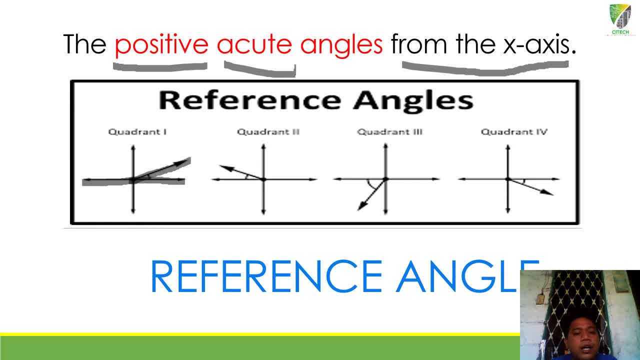 And the terminal side is here And we have here the 30 degrees measurement, Okay, Or given angle. So that is acute angles. Why It is less than 90 degrees or basta, lahat ng less than 90 degrees: 89,, 88,, 87, 86,, 85 hanggang 1 degree. 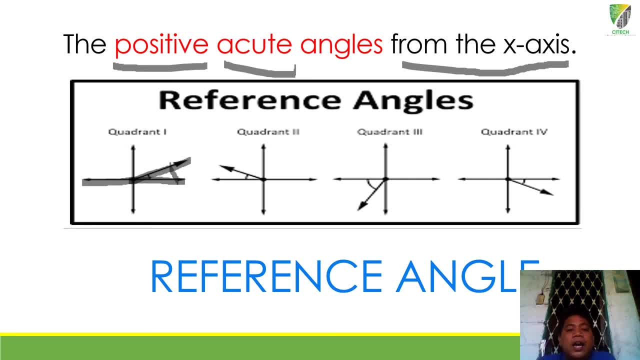 So that is acute angles And it is repairing for reference angles. So quadrant number 1 is a reference angle, Okay, And quadrant number 2, that is also a reference angle. Why, Kasi acute angles siya, Ito, yung angle. 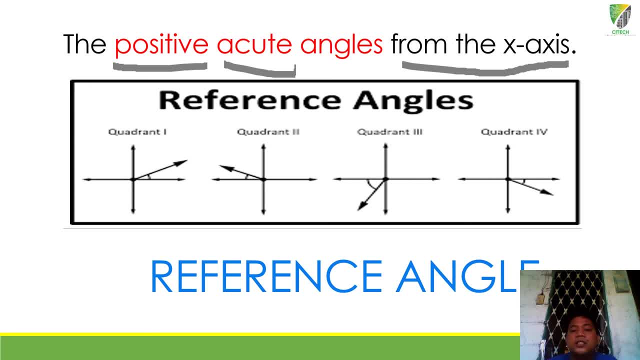 So maybe it is 20 degrees. Next, Quadrant number 3.. So from x-axis going down here. So this is also a positive acute angles. Why This is acute angles? Maybe this is 50 degrees or 45 degrees. 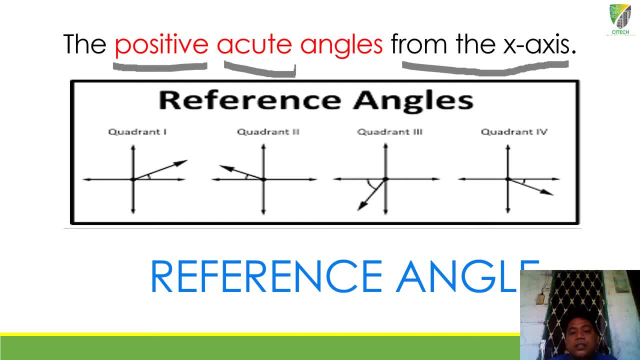 So less than 90 degrees pa rin. So that was reference angle. Okay, So this one. So I think this is 30 degrees. So from x-axis pa rin naman yung kanyang angle into terminal side. This is also a positive acute angles or the reference angle. 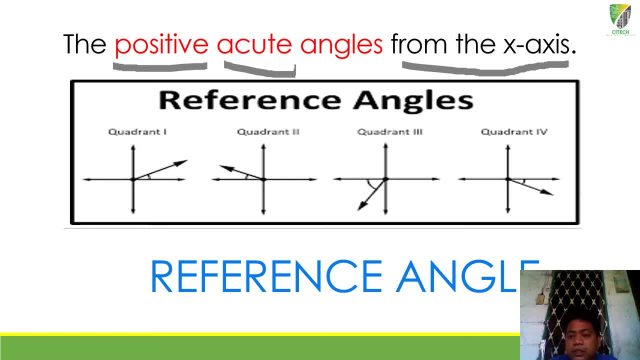 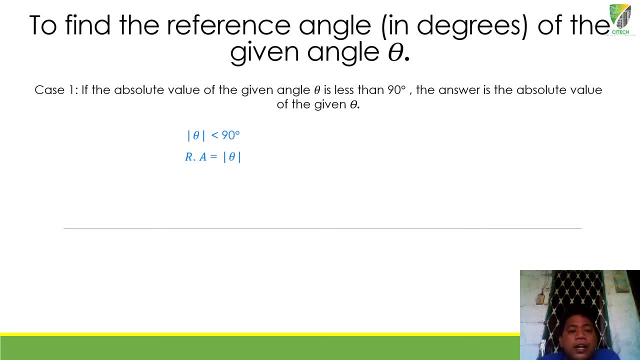 Next, We have here 5 cases. The first one is if the absolute value of the given angle, theta- is less than 90 degrees. be careful, Okay, Okay. So if the absolute value of the given angle for this word less than 90 degrees, if ever, 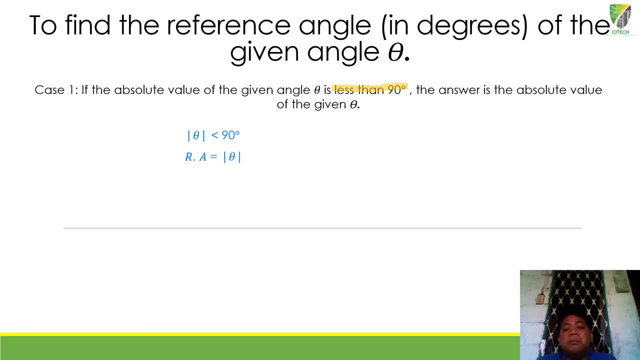 na magnumber tayo ng 91, hindi siya pasok sa case number 1.. O kaya naman okay lang na maging negative to, pero kailangan less than 90 degrees. siya Pasok dyan ng 1 degree to 89 degrees. 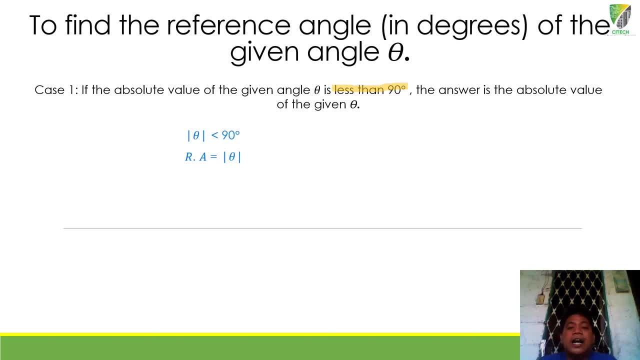 Pero hindi siya lalampas ng 90 degrees. Kailangan less than 90 degrees naman. Okay, So it's less than 90 degrees lang, siya? So again, if the absolute value of the given angle theta is less than 90 degrees, the answer: 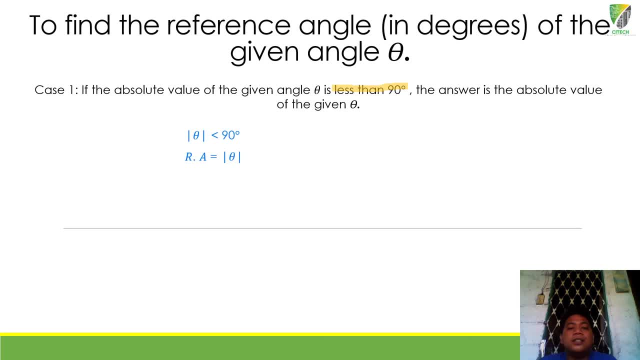 is the absolute value of the given theta. That's it. So ganun lang kabilis Ang mangyayari kapag nalimbawa meron ka man negative, negative 50 degrees. absolute value nyo lang yung negative 50.. 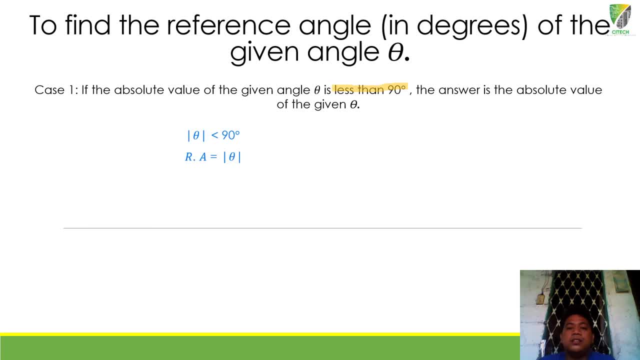 So 50 degrees, Since less than 90 degrees siya pasok na agad siya as the reference angle. Okay, So, like this one. Okay So, for example, Okay So, for example, Okay, Okay, Okay. 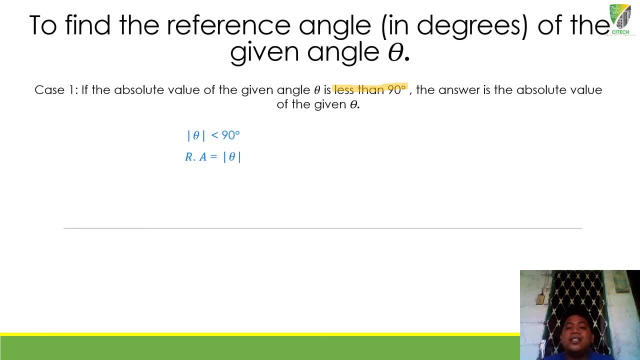 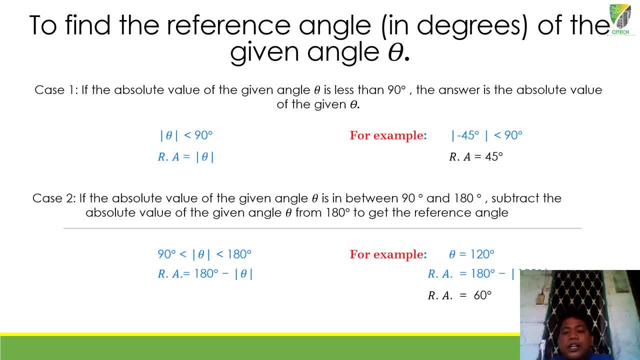 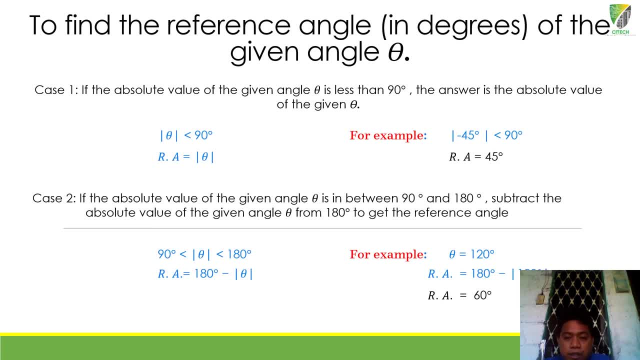 So negative 45 degrees. the absolute value of this is positive 45 degrees. Simply, this is our final answer. Why? Because from the case number 1, or the definition of case number 1, absolute value of the given angle theta is less than 90 degrees. 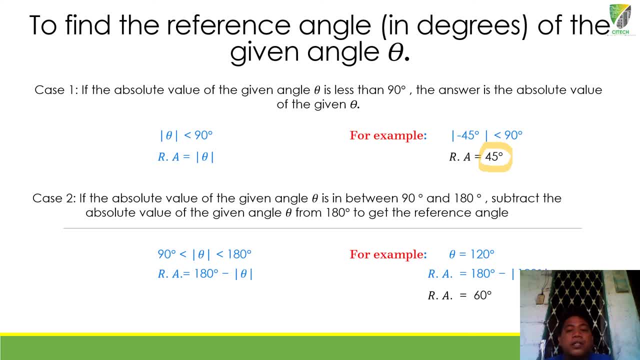 Pasok ba ang negative 45 or positive 45 degrees sa less than 90 degrees? Yes, And the answer is the absolute value of the given theta. That's it. So ito na mismo ang sample. So, kaagad-agad ay, ang reference angle natin na hinahanap ay 45 degrees. 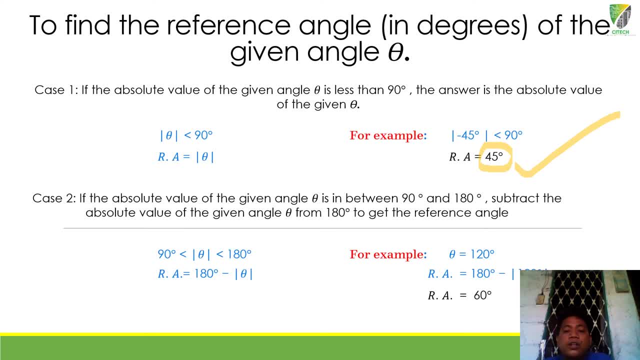 Since, take note ang ating definition for reference angle: positive acute angle. Okay, From the x-axis. So since we have here the positive, So 45 degrees positive acute angle, that is our reference angle. Next, case number 2.. 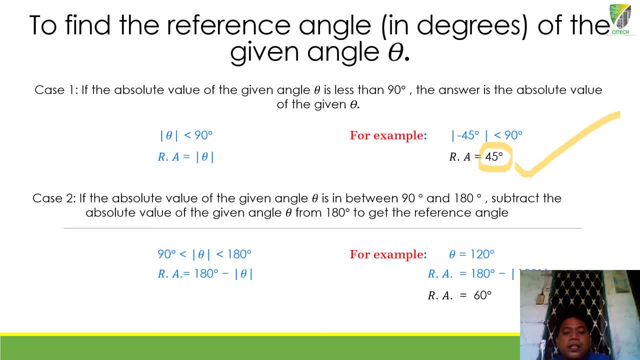 If the absolute value of the given angle theta is in between 90 degrees and 180 degrees, it means that this is in the quadrant 2.. Subtract the absolute value of the given angle theta from 180 degrees to get the reference angle. So we have here. 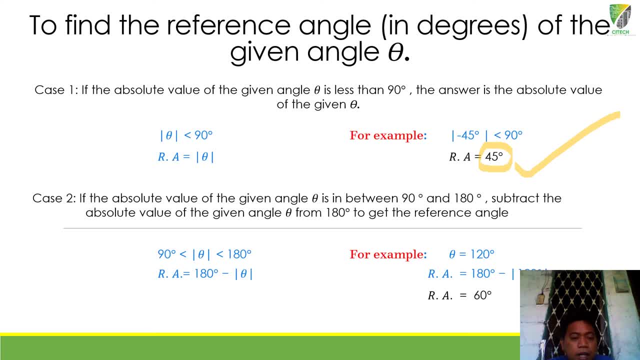 Kailangan maghanap tayo ng given angle, theta natin dito Nasa loob, Nasa loob ng 90 degrees, atsaka ng 180 degrees, For example. we have here A, We have here. 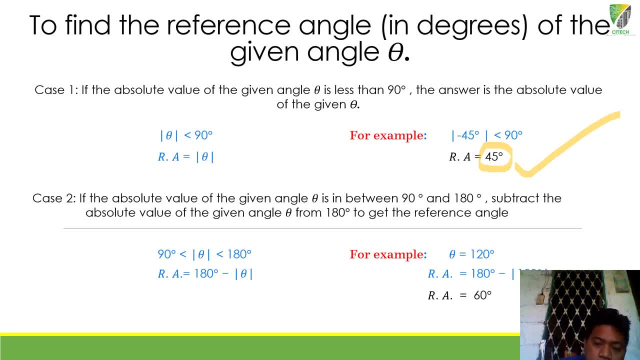 Wait for a while, Maybe you can see the camera. Okay, So we have here the given: Theta is equal to 120 degrees. This is just a given. So theta is equal to 120.. So since we have the formula here to get the reference angle, 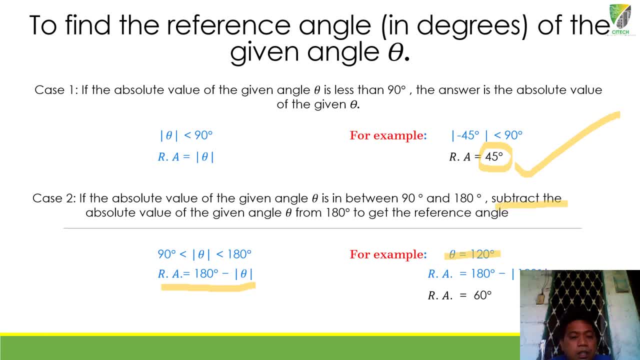 So, according to the definition, subtract the absolute value from the angle theta from 180 degrees, So we have here 180 degrees minus the given angle theta. Okay, So since we have here the given angle theta, 120 degrees, reference angle is equal to 180. 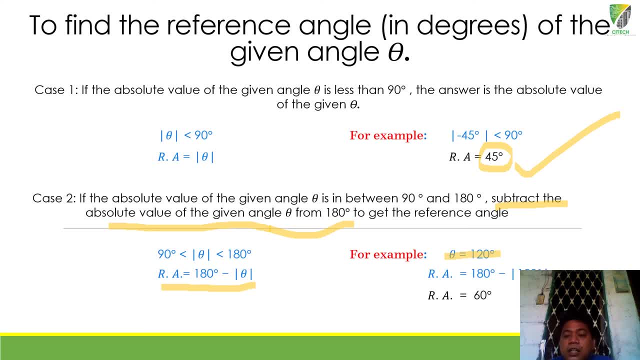 degrees like this one, 180 degrees minus the given, Then angle theta, which is 120 degrees, 180 degrees minus 120 degrees And the answer is 60 degrees, And that's it. That is our reference angle for case number two. 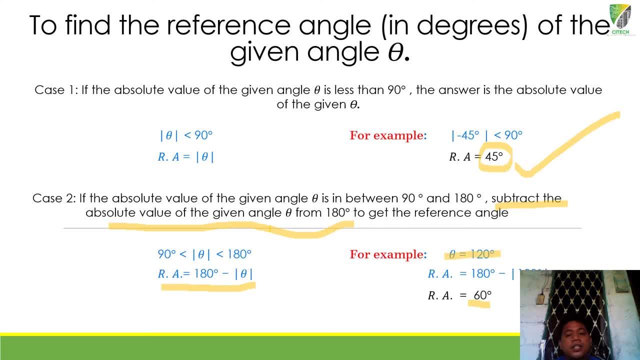 Okay. So, guys, Basta nasa loob sya ng 90 degrees atsaka 180 degrees. Subtract it from 180 degrees and you will find the reference angle. Case number three: If the absolute value of the given angle theta, 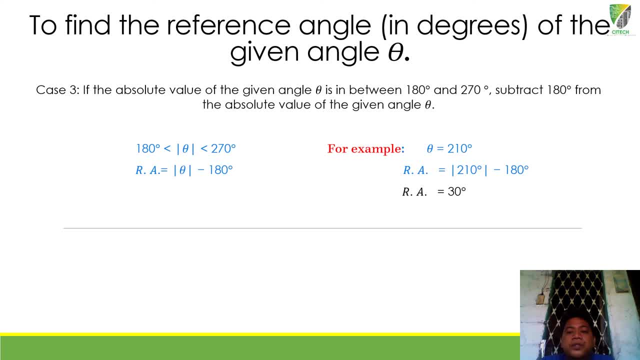 is in between 180 degrees and 270 degrees. subtract 180 degrees from the absolute value of the given angle theta. So medyo may kabaligtaran sya sa case number two dito sa case number three, Why Kanina ang 180 degrees ay nandito sa first term and the theta is here. 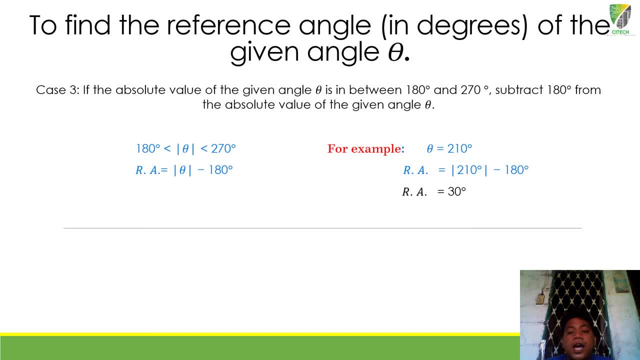 So nagkaroon na lang na pagkakabaligtaran. Pero it's okay, kahit na magkaparehas lang, sila kasi magiging absolute value pa rin naman yung given Kaya wala tayong magiging problem doon. 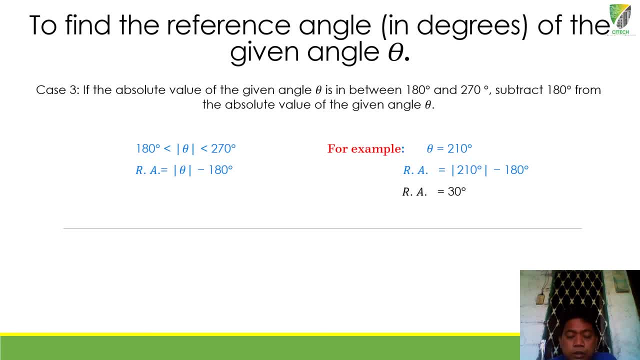 Okay, So theta, for example, sa given natin ay 210 degrees. Okay, So the reference angle is equal to the given. here Let us follow the formula: The given 210 degrees minus 180 degrees and our reference angle is 30 degrees. 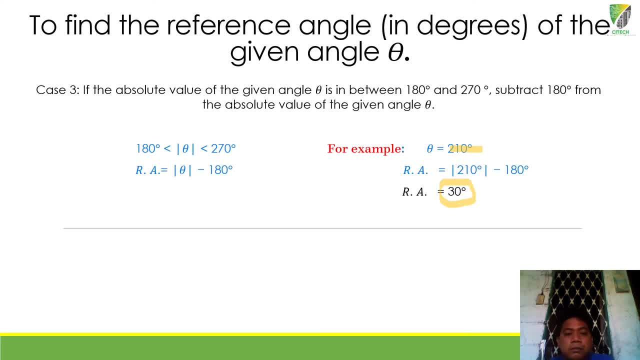 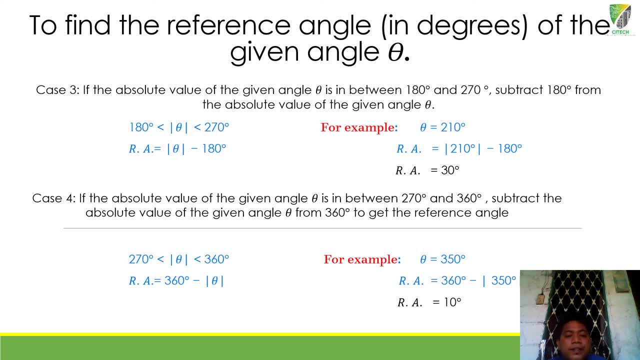 That is positive acute. So it means that is the reference angle. Next, case number four: If the absolute value of the given angle theta is in between 270 degrees and 360 degrees, subtract the absolute value of the given angle theta from 360 degrees to get the reference. 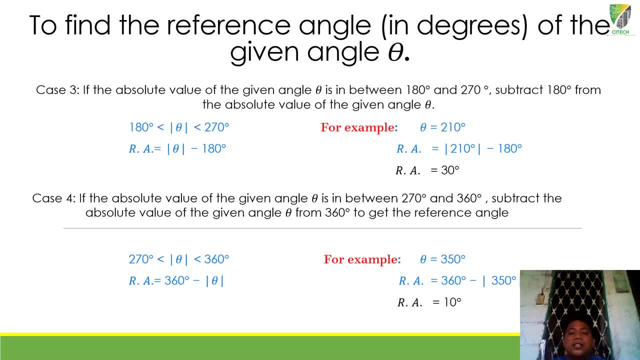 angle. Okay, So dito naman, yung mangyayari naman ay: subtract it from 360 degrees, Ito ay nalang sa quadrant 4 na. So ngayon, here is the given angle: Theta: 350 degrees. 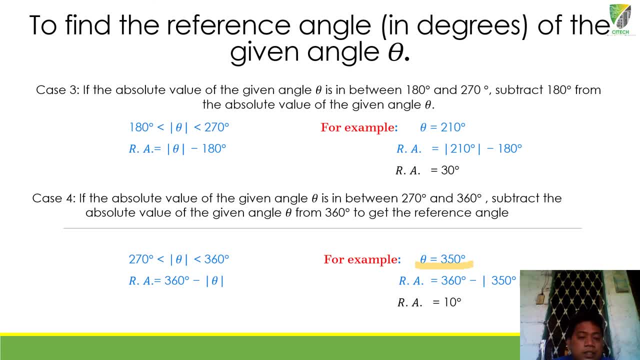 Nagpupol pa rin siya sa 270 degrees, is less than the theta, is less than 360 degrees. Magpupol pa rin siya dito: Mas mataas siya sa 270 degrees, at mas mababa siya sa 360 degrees. 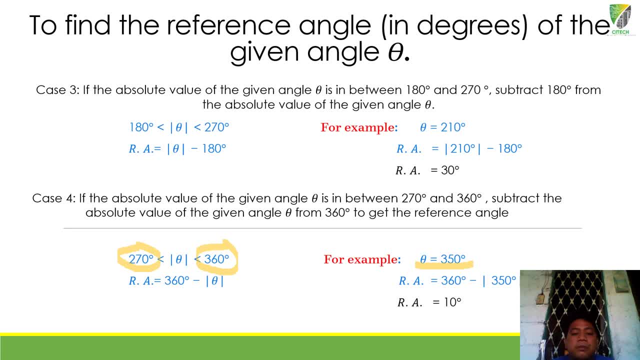 It means pwede na ito sa case number four, Kasi mas mababa Kumbaga nasa gitna siya ng 270 degrees and 360 degrees. So given natin 350 degrees and the formula 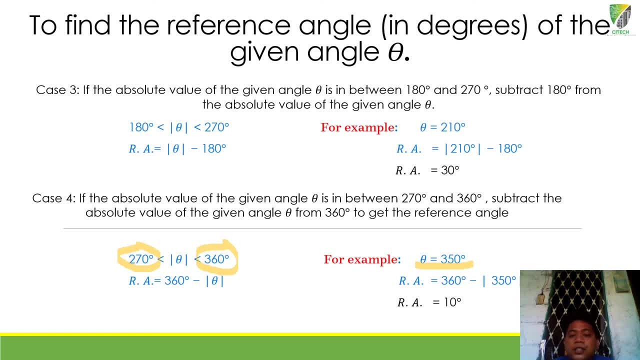 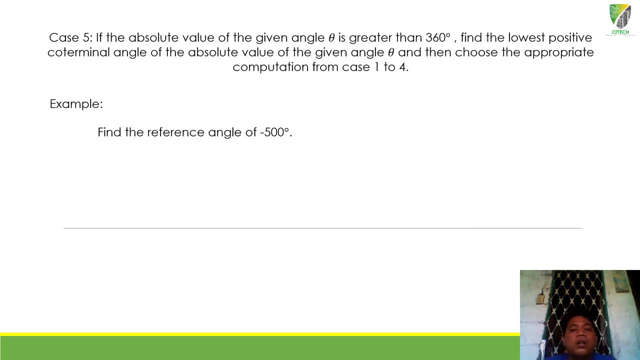 360 degrees minus Minus the given angle theta. So 360 degrees minus 350 degrees and the answer is 10 degrees. So this is a positive acute angle, or what we call the reference angle. Next, last case for our reference angle, we have case number five. 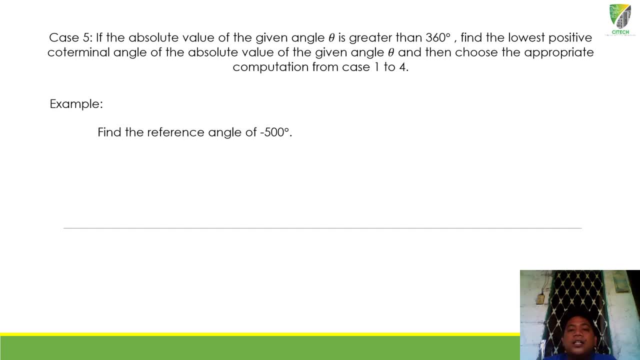 If the absolute value of the given angle theta is greater than 360 degrees. find the lowest positive coterminal angle of the absolute value of the given angle theta And then choose the appropriate computation from case one to four. Okay, so we have here. 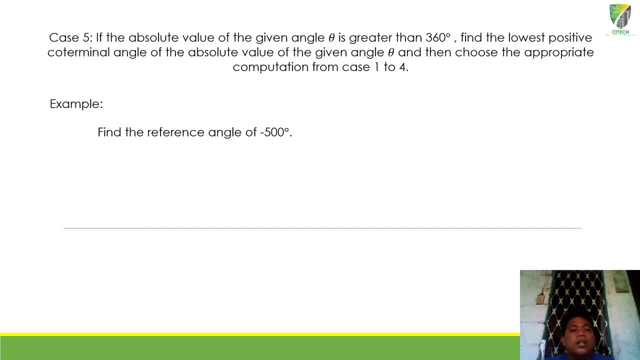 Find the reference angle of negative 500 degrees. Okay, so just be reminded na ang ating given is either negative or positive. It is okay, So walang problema dyan. Why, Kung mapapansin natin? so ito yung solution natin. 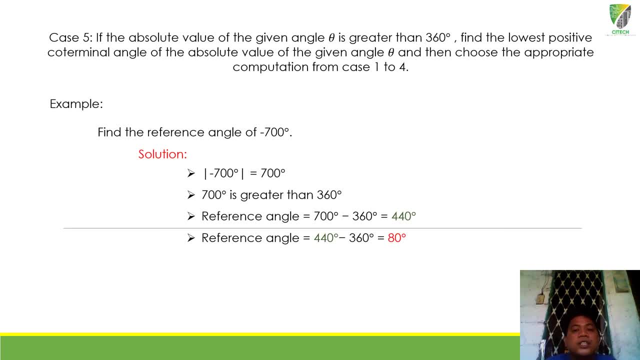 Ay, sorry. So that is negative 700 degrees. Okay, so this is our example: Find the reference angle of negative 700.. Okay, so the first thing you have to do is get first the absolute value of the given. So we have here the negative 700 degrees. 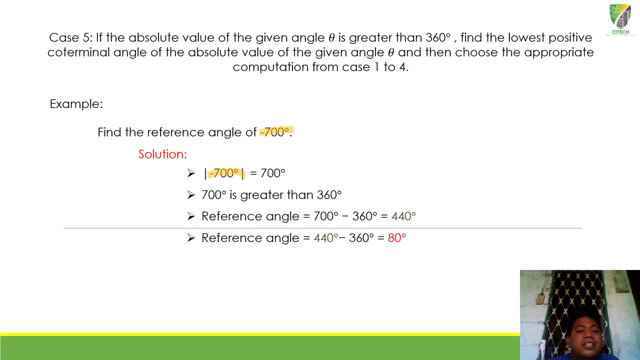 So find the absolute value of negative 700 degrees, So the answer is 700 degrees. So kapag positive naman siya, for example positive 700 degrees, ang sagot pa rin niya ay positive 700 degrees. 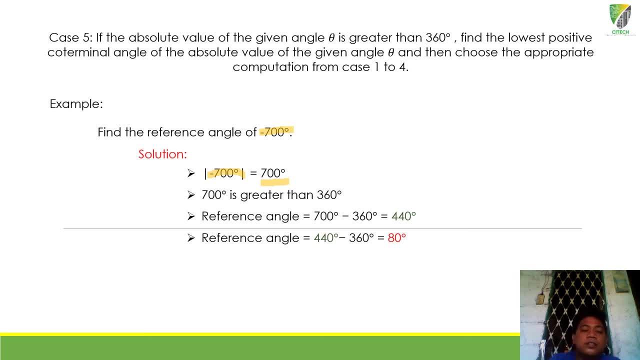 So walang pagbabago dyan. Okay, so Negative man siya, so make it positive para makuha natin yung absolute value. So that is 700 degrees, So next one. the next step is 700 degrees, since it is greater than 360 degrees. 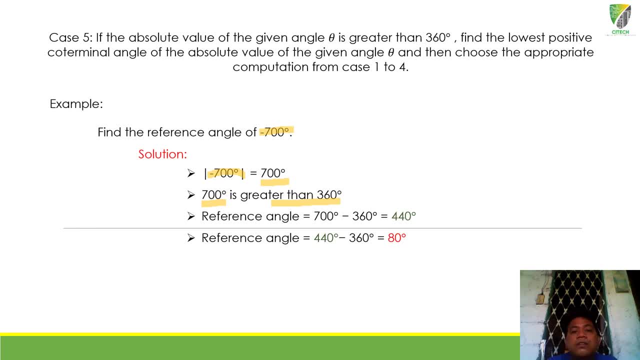 According to the definition, if the absolute value of the given angle theta is greater than 360 degrees, find the lowest positive coterminal angle of the absolute value of the given angle theta and then choose the appropriate computation. So we have here para makuha natin yung reference angle, since alam naman natin yung 700 degrees. 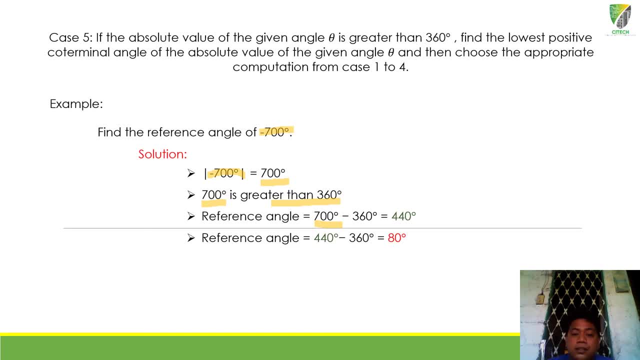 ay mas mataas sa 360 degrees. so just subtract 700 degrees to 360 degrees. Okay, bakit kailangan natin mag-subtract? Kasi kailangan natin makuha yung sinasabi natin na lowest positive coterminal angle. 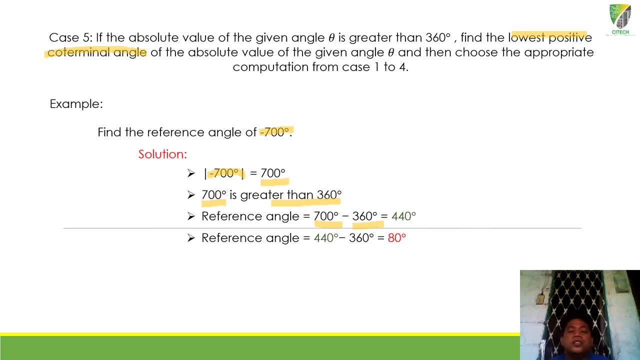 So kailangan makuha natin yung lowest positive coterminal angle. So 700 degrees minus Minus 360 degrees is equal to 440 degrees. So mas mataas pa rin ba ang 440 degrees sa 360?. 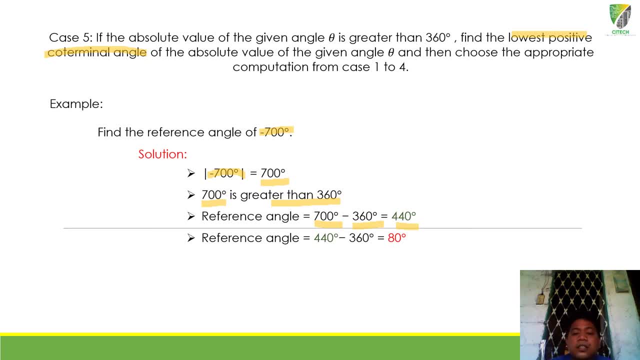 Yes. So ang gagawin lang natin, kung mas mataas pa rin sa 360 degrees. subtract it also from 300, o to 360 degrees, So we have here 440 degrees minus 360 degrees, and the answer is 80 degrees. 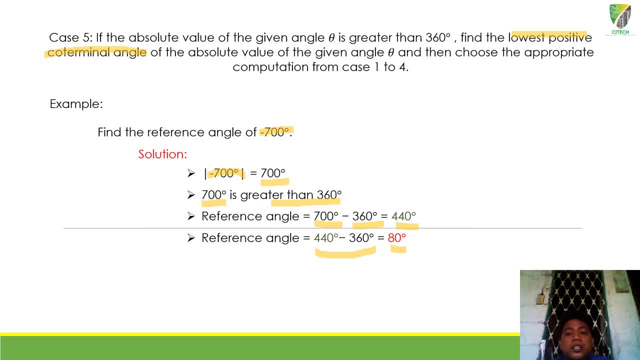 So ngayon ang tanong: 80 degrees ba ay positive acute angle na siya? Yes, Yes, Kung positive acute angle na siya, And that is our answer, or that is our reference angle. Bakit? 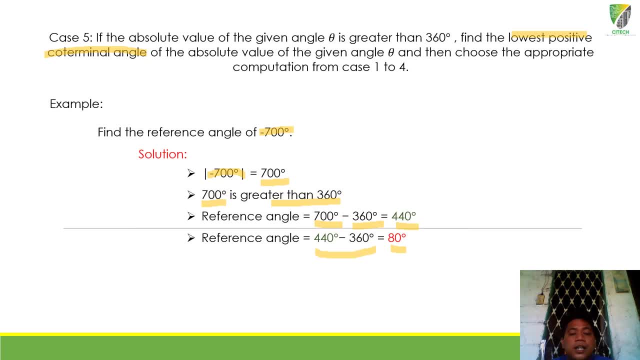 Kasi sabi natin less than 90.. Ang 80 ba ay less than 90?? Yes, So ibig sabihin, pasok siya sa acute angle. Ang 80 degrees ba ay positive? Yes, Kaya, since ang definition natin ng reference angle is positive acute angle, so it means. 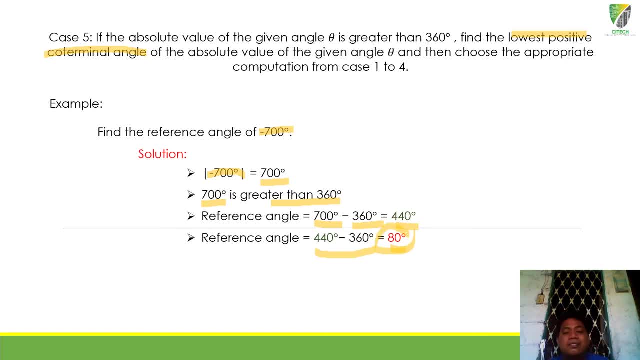 that 80 degrees is our reference angle. Okay, so, guys, thank you very much for listening and for your cooperation. So nawa ay 90 degrees. Thank you for listening and for understanding our topic. the key concepts: the first one: 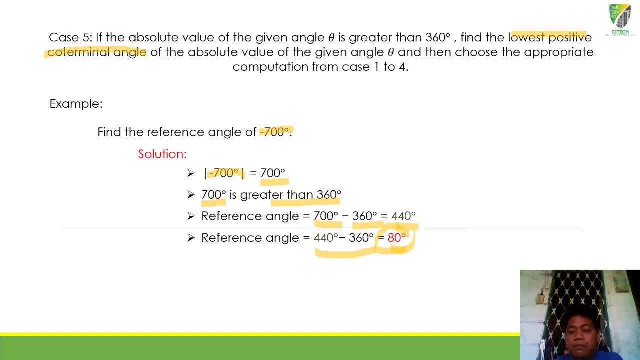 and the second one is the coterminal angles and the third one is the reference angle. Thank you and have a nice day.